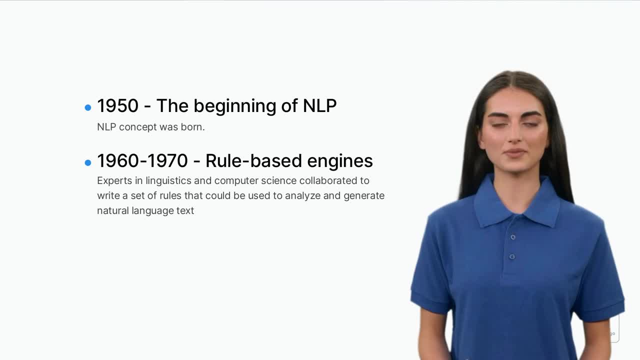 linguistics and computer science collaborated to write a set of rules that could be used to analyze and generate natural language text. however, these rule-based systems were limited in their ability to handle complex language tasks and required significant manual effort to develop. in the 1980s, researchers began exploring statistical approaches to 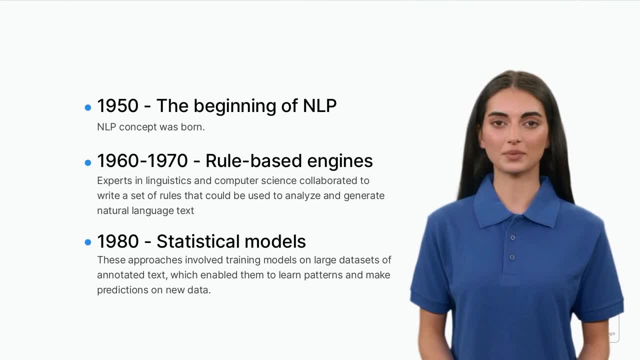 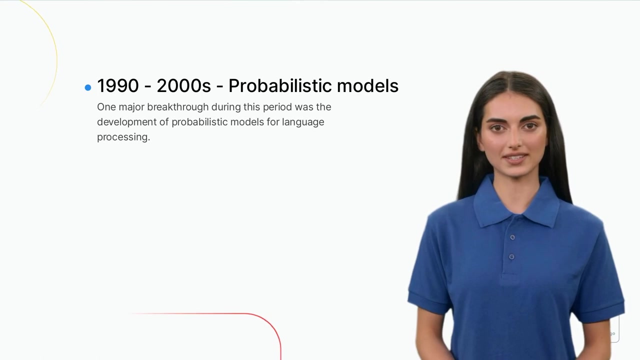 nlp. these approaches involved training models on large data sets of annotated text which enabled them to learn patterns and make predictions on new data. this shift towards statistical methods led to significant advances in machine translation, speech recognition and other nlp applications. in the 1990s and 2000s, researchers continued to refine statistical and machine 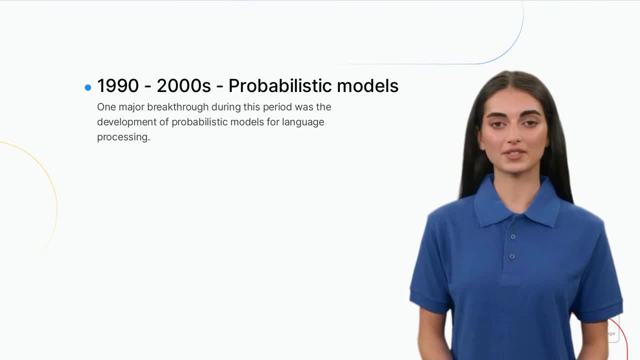 learning approaches to nlp. one major breakthrough in nlp research was the introduction of the nlp text to nlp. code grows to be more accessible using a more complex language processing model such as hidden markov models and conditional random fields. these models improved the accuracy of nlp. 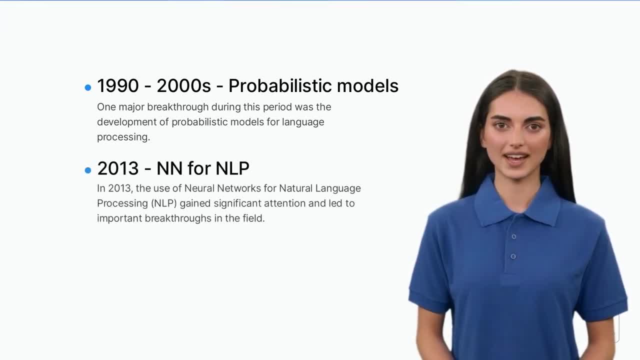 systems and enabled them to handle more complex language tasks. in 2013, the use of neural networks for natural language processing- nlp- gained significant attention and led to important breakthroughs in the field. one key development was the introduction of a new nlp text-based training. 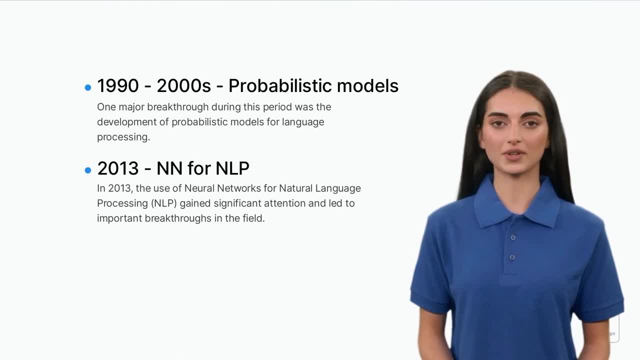 of the word-to-vec algorithm, which uses neural networks to learn distributed representations of words in a corpus of text. This approach allowed words with similar meanings to be represented as similar vectors in a high-dimensional space, enabling NLP models to better capture semantic. 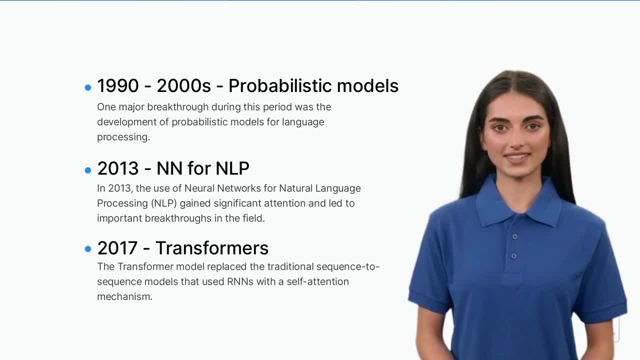 relationships between words. In 2017, the Transformer network was introduced as a new neural network architecture for natural language processing, NLP. The Transformer was proposed in a paper titled Attention is All You Need by Veswani et al. The Transformer model replaced. 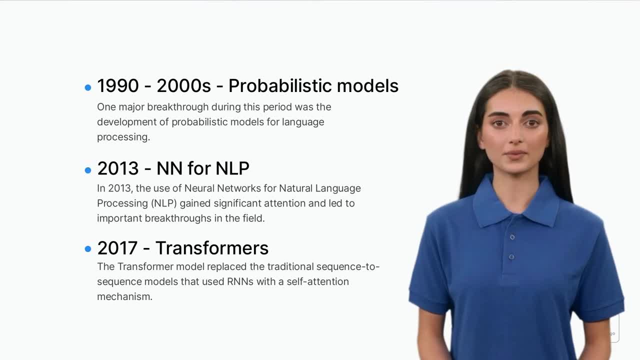 the traditional sequence-to-sequence models that used recurrent neural networks, RNNs- with a self-attention mechanism. This mechanism allows the model to process input sequences in parallel rather than sequentially, making it more efficient and effective for handling longer input sequences.